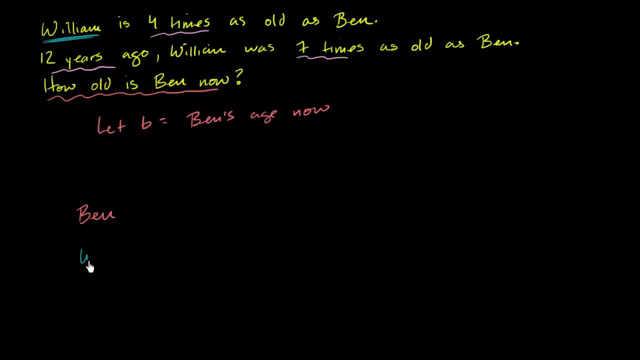 And then let's think about William. I'll do William in blue here. So let's think about William. And then there's two points in time we're talking about. We're talking about now, today, and we're going to talk about 12 years ago. 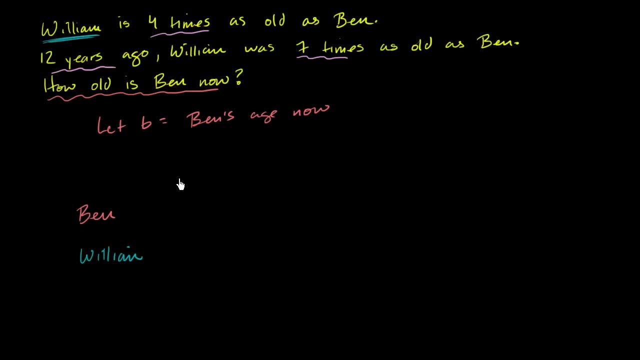 So let's talk about over here, Let's say today, or let's call that now, This will be our now column and then this will be our 12 years ago. So let's see what we can fill in here. So what is Ben's age now? 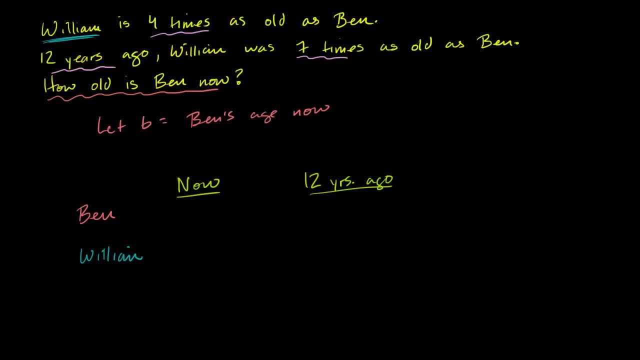 Well, we just defined that as the variable b, That's the unknown. That's what we have to figure out, So let's just stick that there. So that's just going to be b. Well, what's Ben's age 12 years ago? 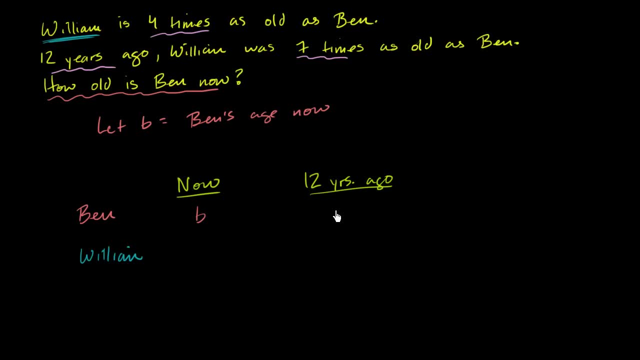 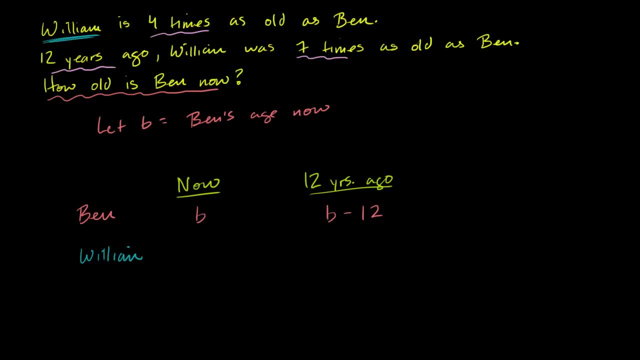 That's b minus 12.. Fair enough, Now, what is William's age today? Well, this first sentence gave us the information: William is four times as old as Ben, And we can assume that they're talking about today. Is is four times as old as Ben. 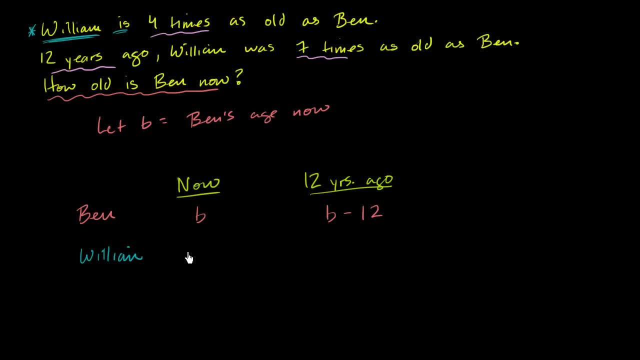 So if Ben is b, William is going to be 4b, And so how old was William 12 years ago? Well, if he's 4b Right now, 12 years ago, he'll just be 12 less than that. 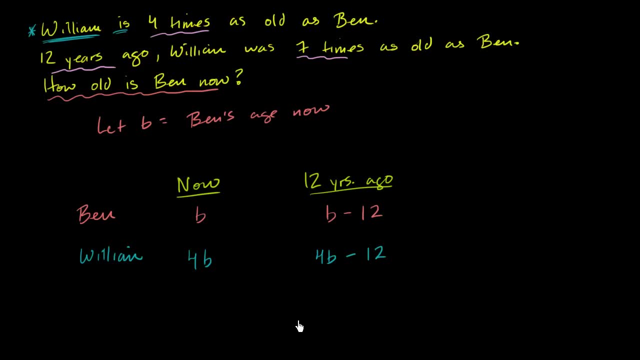 So he's 4b now. 12 years ago it was 4b minus 12.. So that's kind of interesting, But we haven't quite yet made use of this second statement 12 years ago, William. So this is William 12 years ago. 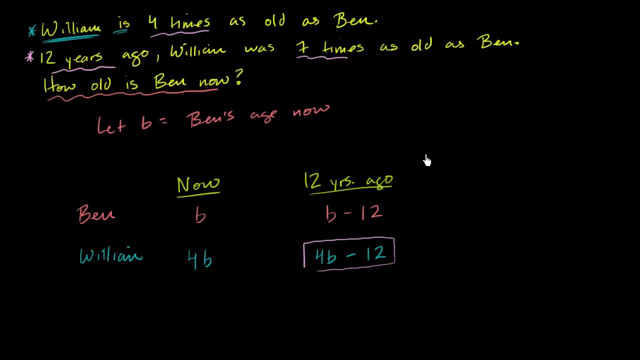 12 years ago, William was seven times as old as Ben. So 12 years ago this number is going to be seven times this number, Or another way to think about it: take this number and multiply it by seven And you're going to get this number. 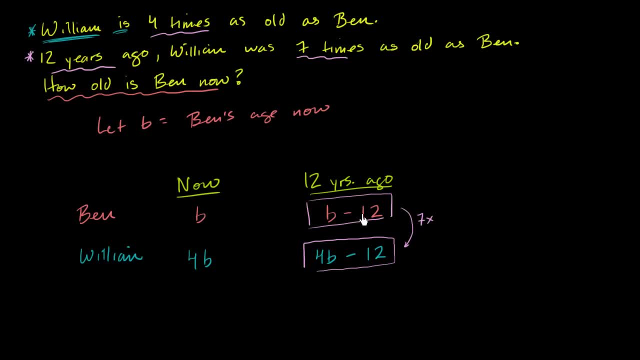 12 years ago. Ben's age is 1 seventh of William's age, Or William's age is seven times Ben's age. So let's see if we can set that up as an equation. So we can have seven times this. Let me write this down. 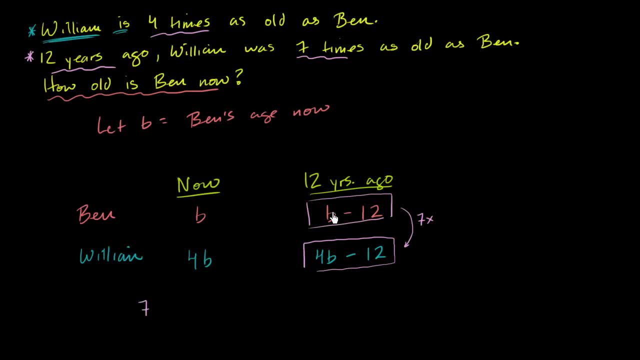 Seven times Ben's age 12 years ago, Seven times 10.. And Ben's age 12 years ago, b minus 12, is going to be equal to William's age, And it seems like we've done the hard part. We've set up the equation. 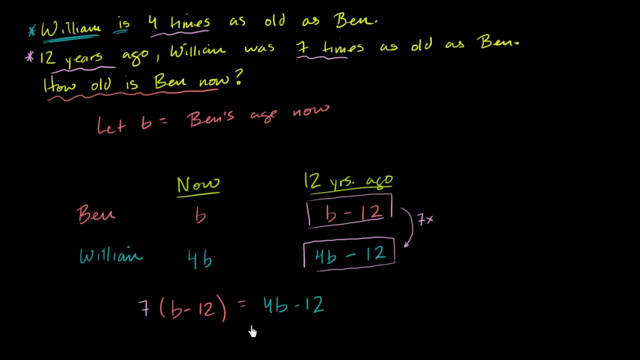 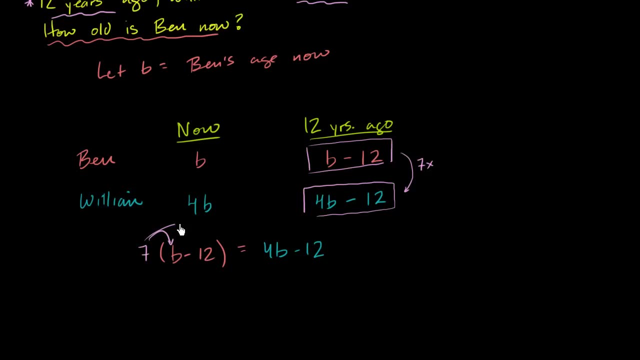 Now we just use a little bit of our algebraic tools to solve for b. So let's do that. So the first thing we might want to do, we could distribute this: 7.. So 7 times b, 7 times essentially negative, 12.. 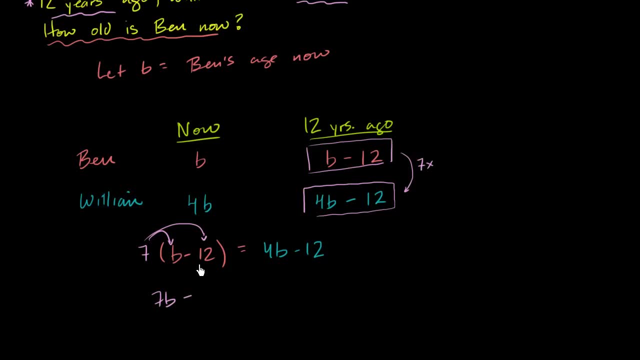 So we have 7b minus 12.. Minus 7 times 12. Let's see it's 84.. 84 is going to be equal to 4b minus 12.. This whole expression is literally seven times Ben's age 12 years ago. 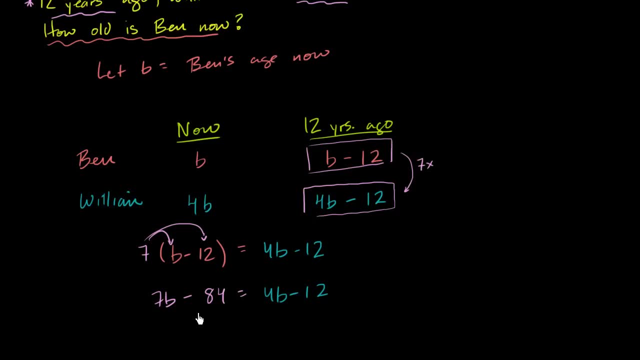 Now, what can we do to solve this? Well, we can subtract 4b from both sides. So let's do that 4b. I can do two steps at the same time. Well, actually, Let's just keep it simple. 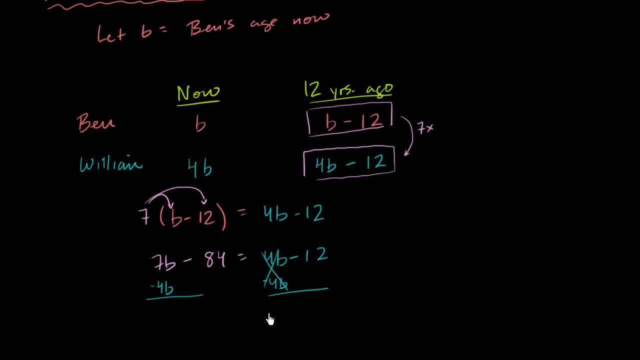 So I'm going to subtract 4b from both sides. That goes away. On the right-hand side I have a negative 12.. On the left-hand side, I'm left with 7b. minus 4b is 3b. 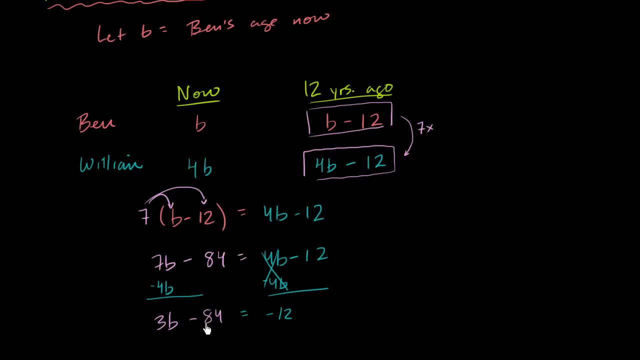 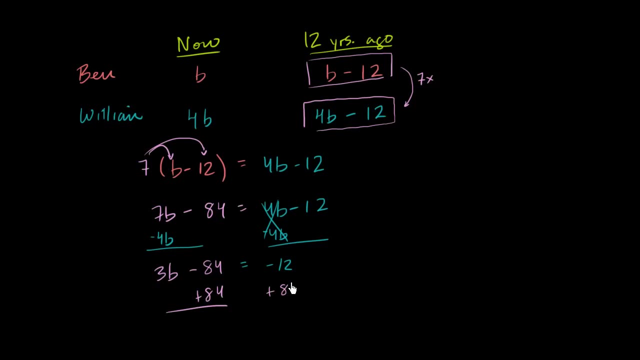 And then I still have a minus 84.. Well, I want to get rid of this negative 84, this minus 84 on the left-hand side. So let's add 84 to both sides. On the left-hand side, I'm just left with 3b. 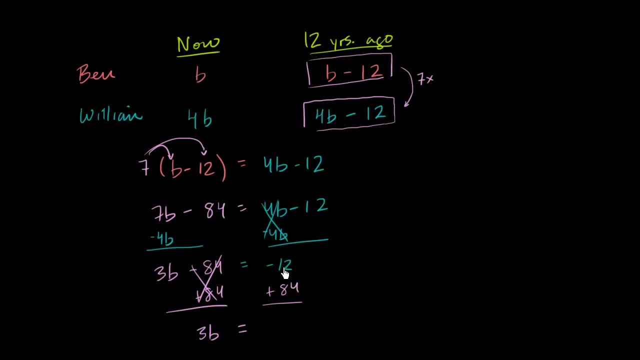 And on the right-hand side I have negative 12 plus 84.. Or 84 minus 12, which is 72.. 72. Now if I want to solve for b, I just have to divide both sides of that equation by 3.. 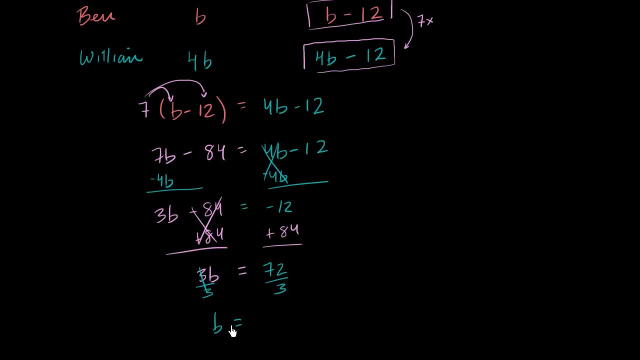 And so I am left with. b is equal to- and now we have our drum roll- 72 divided by 3. And you might be able to do that in your head. It would be 24,, I believe, And you could work it out on paper if you have trouble. 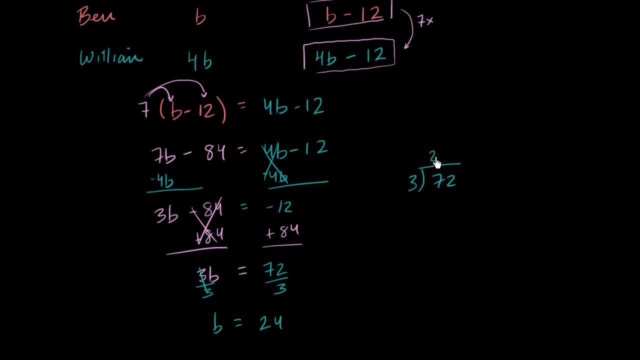 Let's just do it real quick: 72.. 3 goes into 7 two times. Then you get a 7. You get a 2 times 3 is 6.. Subtract, You bring down the 2. 3 goes into 12 four times.